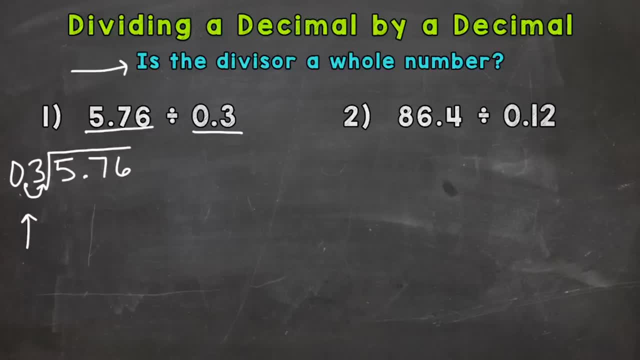 the ones place, So moving the decimal once to the right, or you can think of it as sliding the 3 over to the ones place. we multiplied that outside number by 3 tenths, So we can do this by number by 10.. So if you do something to the outside number, that divisor, you have to do. 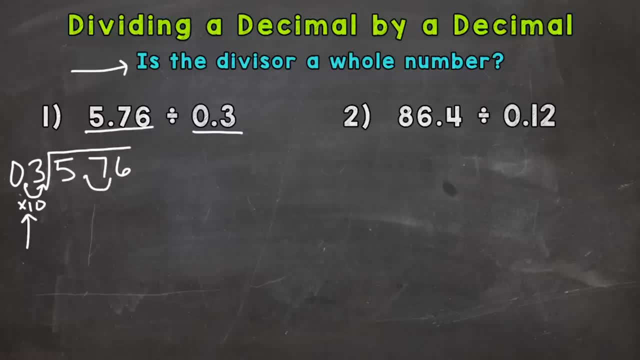 the same thing to the inside. Remember, whatever you do to the outside, you have to do to the inside. So we moved the decimal once to the right and therefore shifted each digit one spot to the left. Let's do the same thing to the inside. the dividend: Now we're ready to go as far as setting 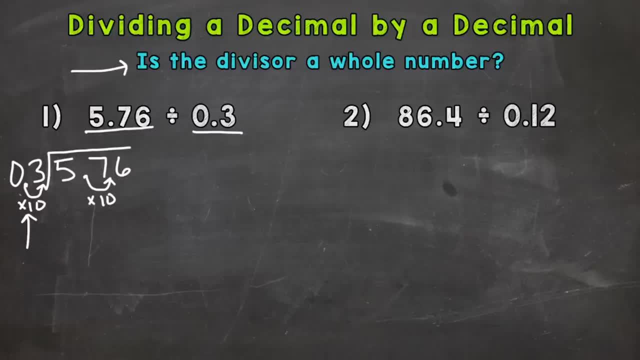 up our problem with a whole divisor. So we have those arrows underneath there. so let's rewrite our problem so it's a little more neat. So we have 3 as our divisor and for our dividend we have 57 and 6 tenths. So now is our divisor whole. Yes, we can start our problem So. 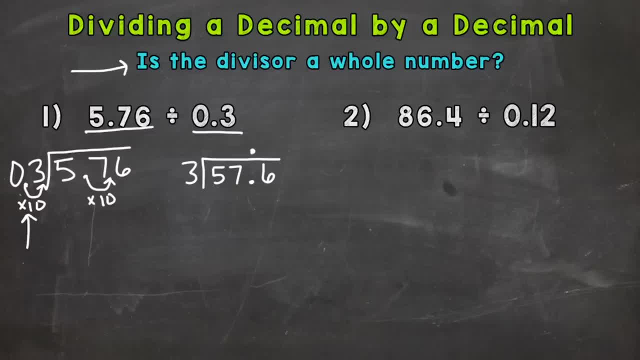 once your divisor is whole, you bring your decimal straight up and go through your division process. So divide, multiply, subtract, bring down and repeat. So 5 divided by 3, how many whole groups of 3? 5 divided by 3, how many whole groups of 3? 5 divided by 3, how many whole groups of 3?? 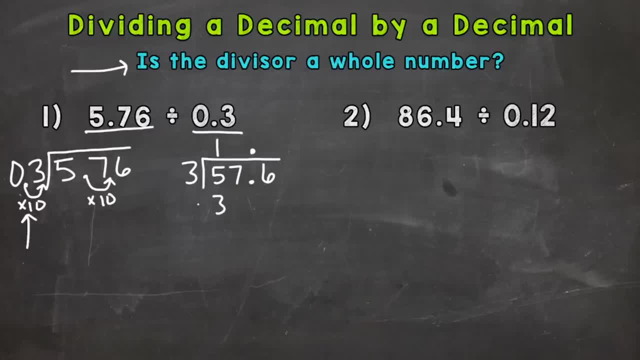 3 out of 5? Well, 1.. 1 times 3 is 3.. Subtract: we get 2.. Bring down the 7.. 27 divided by 3 is 9.. 9 times 3, 27.. Subtract: we get 0.. Bring down this 6 here, And we end with 6 divided by 3, which is 2.. 2 times 3 is 6.. Subtract, and we get a. 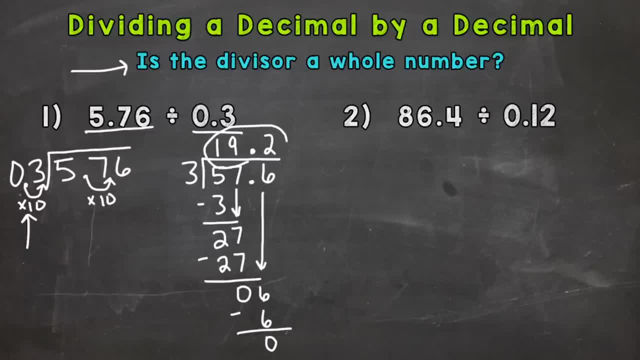 clean cut 0 here and a final answer of 19 and 2 tenths. So let's do another example here in order to get this down a little better, And number 2 is going to be a little different, and you'll see why. 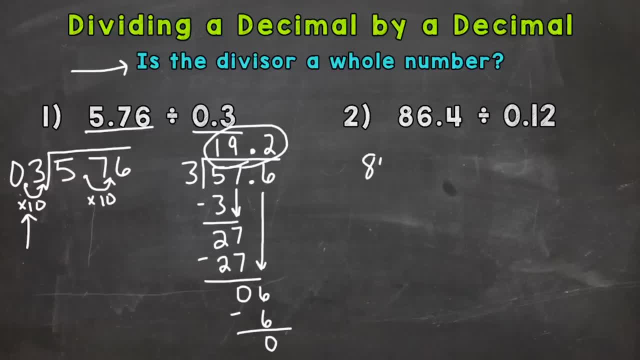 here in a second. So our dividend 86 and 4 tenths is the number being divided or split up and that goes underneath the division bar. So 86 and 4 tenths divided by 12 hundredths, So 12 hundredths. 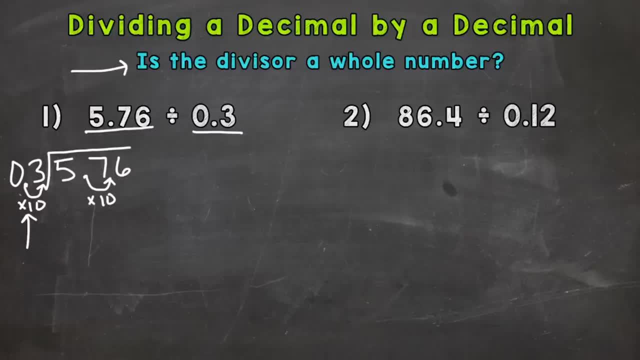 up our problem with a whole divisor. So we have those arrows underneath there. so let's rewrite our problem so it's a little more neat. So we have 3 as our divisor and for our dividend we have 57 and 6 tenths. So now is our divisor whole. Yes, we can start our problem So. 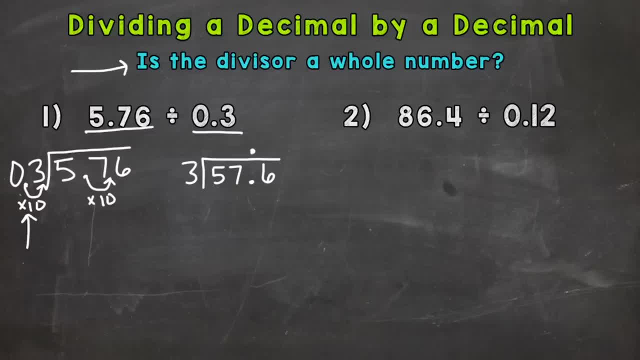 once your divisor is whole, you bring your decimal straight up and go through your division process. So divide, multiply, subtract, bring down and repeat. So 5 divided by 3, how many whole groups of 3? 5 divided by 3, how many whole groups of 3? 5 divided by 3, how many whole groups of 3?? 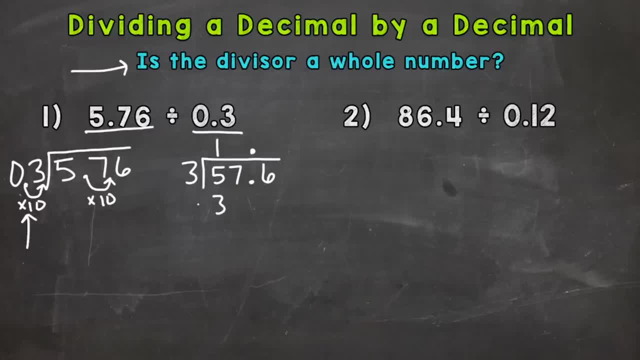 3 out of 5? Well, 1.. 1 times 3 is 3.. Subtract: we get 2.. Bring down the 7.. 27 divided by 3 is 9.. 9 times 3, 27.. Subtract: we get 0.. Bring down this 6 here, And we end with 6 divided by 3, which is 2.. 2 times 3 is 6.. Subtract, and we get a. 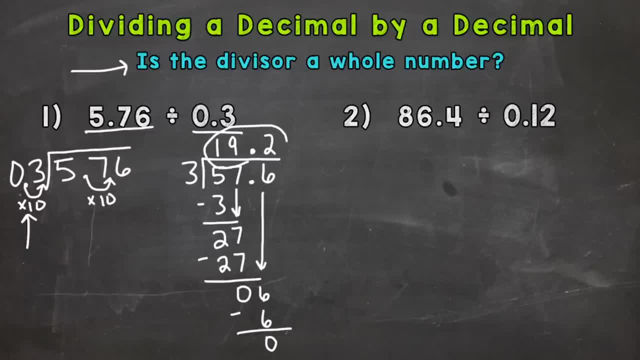 clean cut 0 here and a final answer of 19 and 2 tenths. So let's do another example here in order to get this down a little better, And number 2 is going to be a little different, and you'll see why. 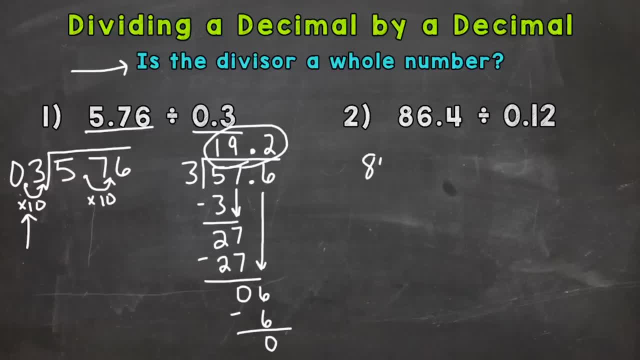 here in a second. So our dividend 86 and 4 tenths is the number being divided or split up and that goes underneath the division bar. So 86 and 4 tenths divided by 12 hundredths, So 12 hundredths. 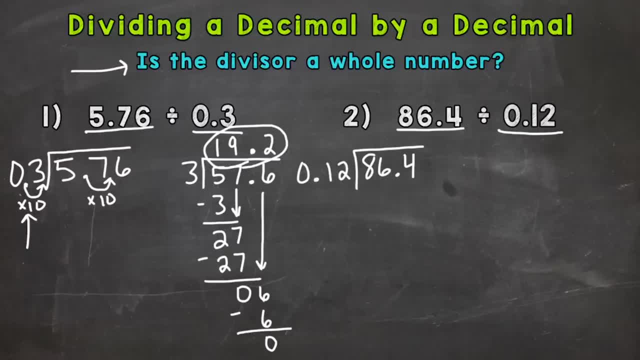 is our divisor. It goes on the outside. Now let's ask ourselves the important question: Is the divisor a whole number? No, So we need to make it a whole number in order to go through the process. So let's multiply by a power of 10.. Let's multiply by 10, and now the decimal will be between the 1. 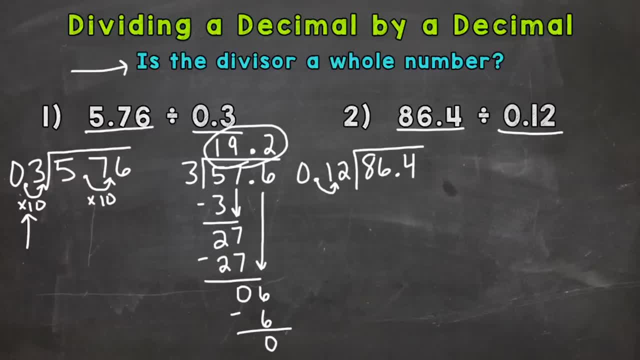 and the 2.. Is that a whole number? No, So we need to multiply by 10 again, So 10 times 10.. We need to multiply that. We need to multiply the outside number by 100 in order to push the digits to the correct place values in order. 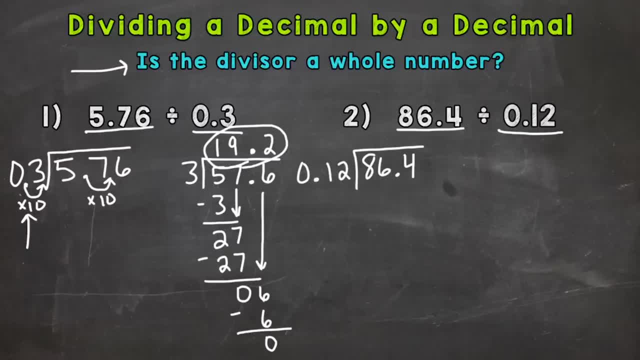 is our divisor. It goes on the outside. Now let's ask ourselves the important question: Is the divisor a whole number? No, So we need to make it a whole number in order to go through the process. So let's multiply by a power of 10.. Let's multiply by 10, and now the decimal will be between the 1. 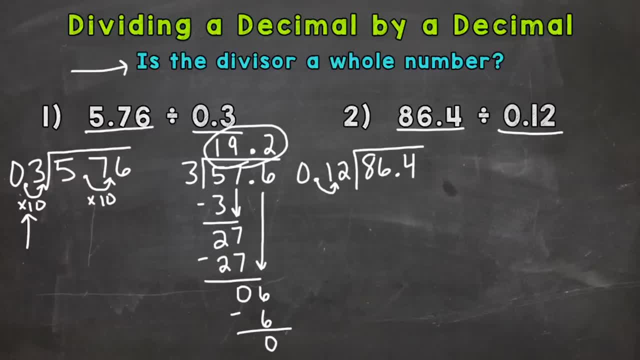 and the 2.. Is that a whole number? No, So we need to multiply by 10 again, So 10 times 10.. We need to multiply that. We need to multiply the outside number by 100 in order to push the digits to the correct place values in order. 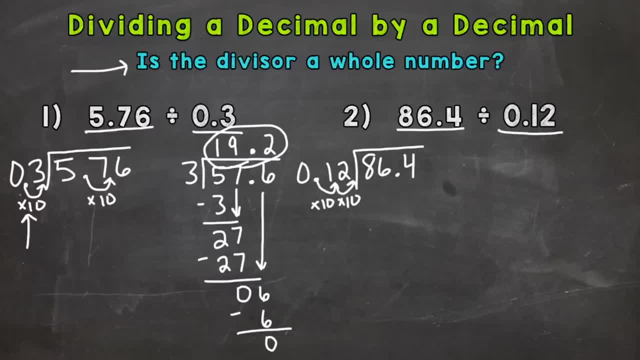 to make it a whole number. So we need to move the decimal twice, or multiply that 86 and 4 tenths by 100 as well. Remember, whatever you do to the outside, you do to the inside. So once, twice and we can fill that with a. 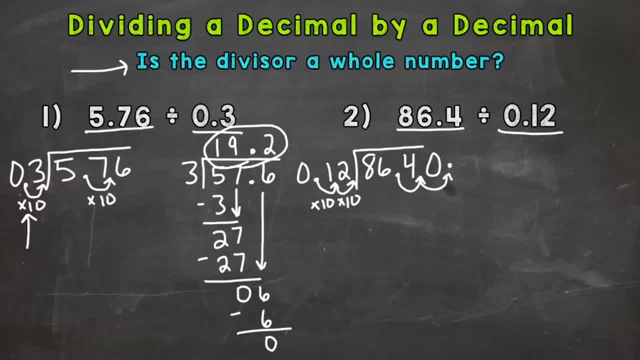 placeholder 0 there And our decimal goes at the end. So now we actually have a whole dividend. So our new problem is going to be 12.. And on the inside our dividend is 8640. And that decimal is at the end. So we don't really need it when it comes to. 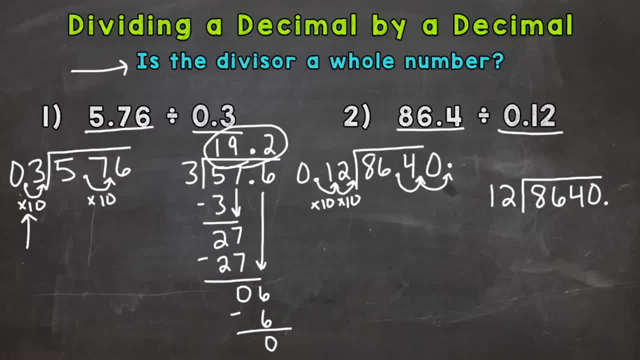 whole numbers. but we can put it there in case we need to extend with zeros for remainder purposes. So we'll see if we'll need that decimal as we go through this problem. So let's go through our steps. So 8 divided by 12.. Well, we can't pull any whole groups of 12 out of 8. So we need to go to 86.. So how many whole groups of 12 out of 86?? 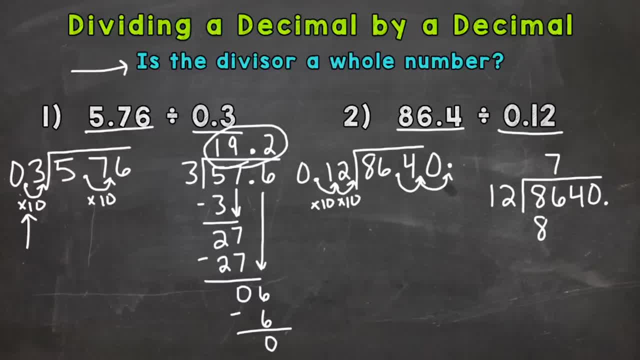 Well, 7 times 12 is 84.. That's as close as we are going to get. So 7.. 7 times 12 is 84.. Subtract, We get 2.. Bring down the 4.. So 24 divided by 12.. 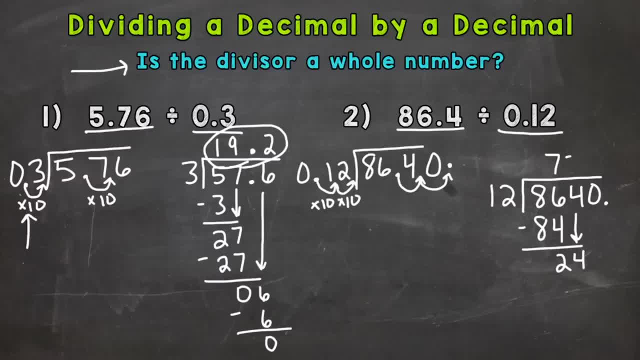 How many whole groups of 12 out of 24?? Well, 2. 2 times 12 is 24.. subtract we get 0.. Now do not stop here. We did not go all the way over to the ones place here. 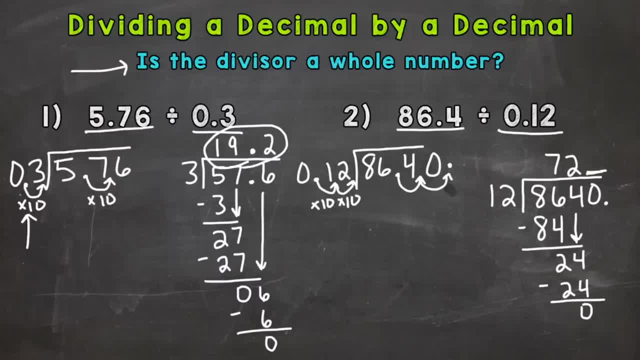 so our answer is not 72.. We need to keep going because we still have numbers to bring down here. So let's bring our 0 down and we have 0 divided by 12.. So how many whole groups of 12 out of 0?? 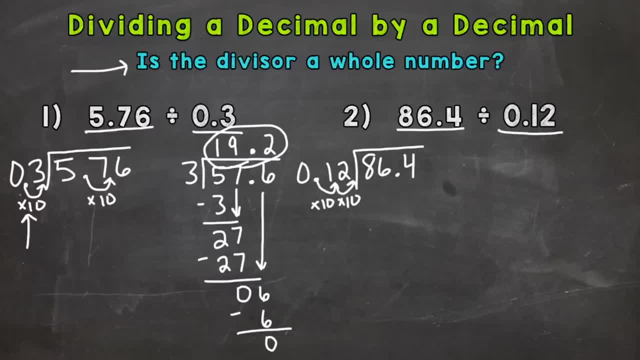 to make it a whole number. So we need to move the decimal twice, or multiply that 86 and 4 tenths by 100 as well. Remember, whatever you do to the outside, you do to the inside. So once, twice and we can fill that with a. 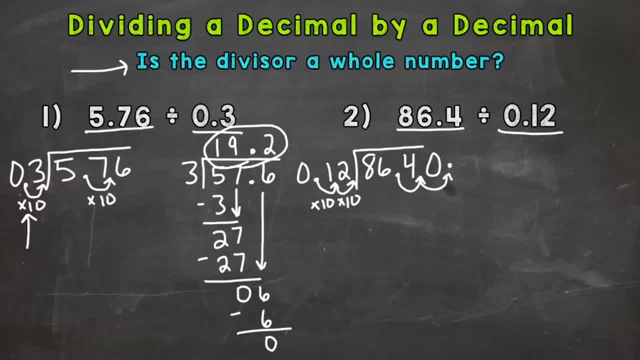 placeholder 0 there And our decimal goes at the end. So now we actually have a whole dividend. So our new problem is going to be 12.. And on the inside our dividend is 8640. And that decimal is at the end. So we don't really need it when it comes to. 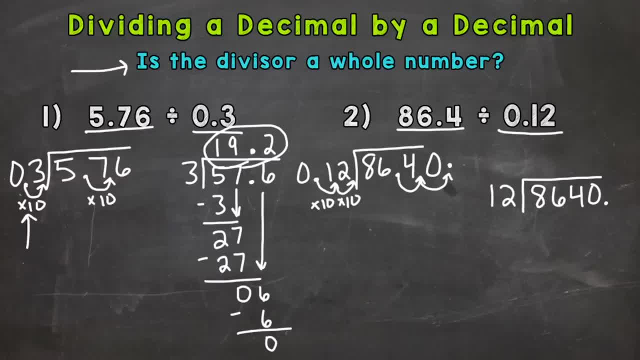 whole numbers. but we can put it there in case we need to extend with zeros for remainder purposes. So we'll see if we'll need that decimal as we go through this problem. So let's go through our steps. So 8 divided by 12.. Well, we can't pull any whole groups of 12 out of 8. So we need to go to 86. So how many whole? 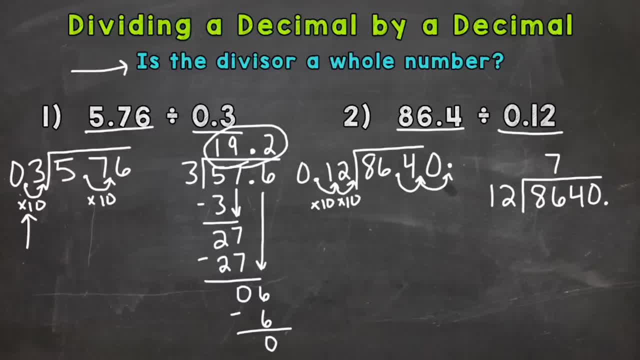 groups of 12 out of 86?? Well, 7 times 12 is 84. That's as close as we are going to get. So 7. 7 times 12 is 84. Subtract, We get 2.. Bring down the 4.. So 24 divided by 12.. How many whole groups of 12 out of 24?? Well, 2. 2 times 12 is. 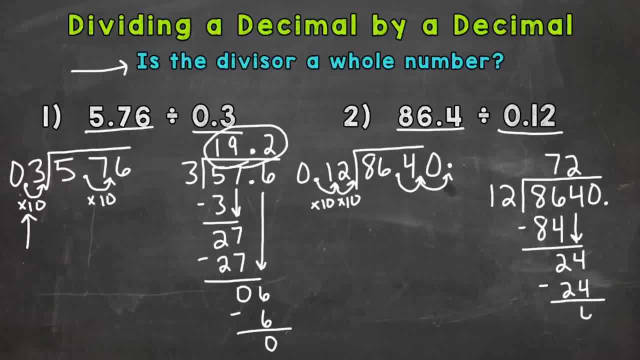 24.. subtract, we get 0. now, do not stop here. we did not go all the way over to the ones place here, so our answer is not 72. we need to keep going because we still have numbers to bring down here. so let's bring our 0 down. and we have 0 divided by 12. so how many whole groups of 12 out of 0? well, 0, 0 times. 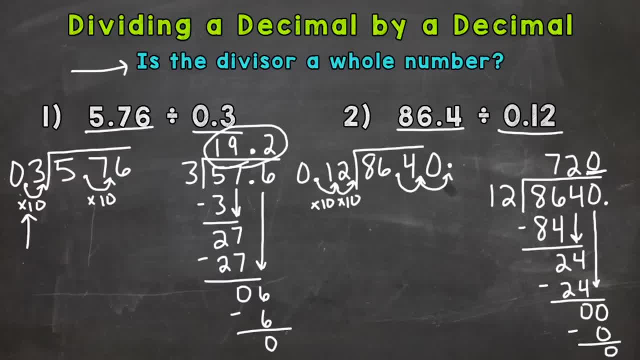 12 is 0 subtract and we get 0, so remember our decimals at the end there. so it's just a whole number and our final answer is going to be 720. so there you have it. there's how you divide a decimal by a decimal. remember: is the divisor a whole number? if not, we need to multiply it by a power.